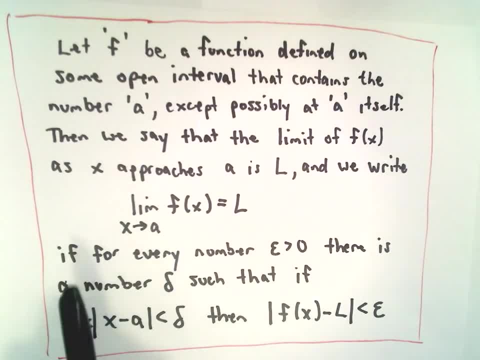 I'm sure you've seen this: The limit as x approaches a of f of x equals l. Okay, here's the technical part that kind of bothers people. If for every number epsilon greater than zero there's a number delta, such that if the absolute value of x minus a is greater than zero and less than delta, 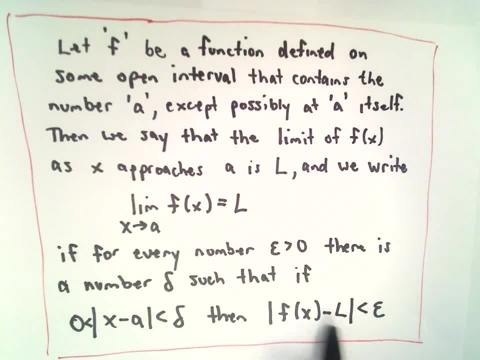 then the absolute value of the quantity f of x minus l is less than epsilon. What the heck does that last part mean? Okay, so again, intuitively, let's take a quick little example. All right, so here's my function: f of x. 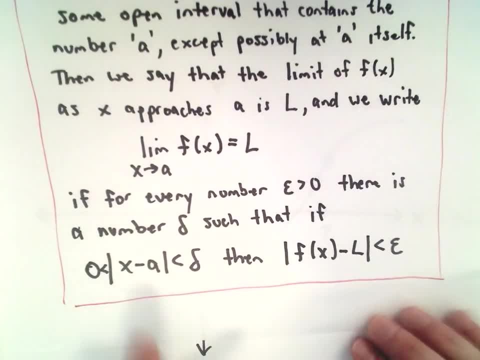 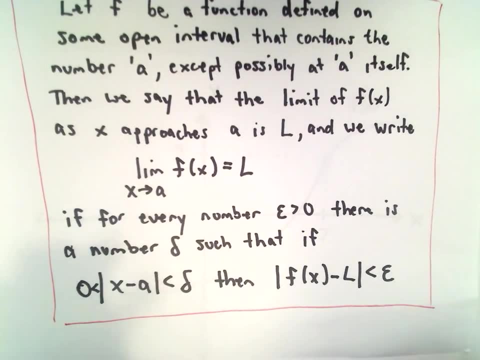 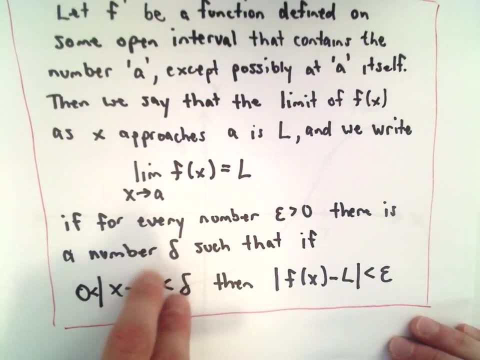 What this definition is trying. the stuff at the bottom. it's trying to formalize the notion of closeness, of being close to something, And we'll talk about these absolute value inequalities in just a second. That's all it's saying. 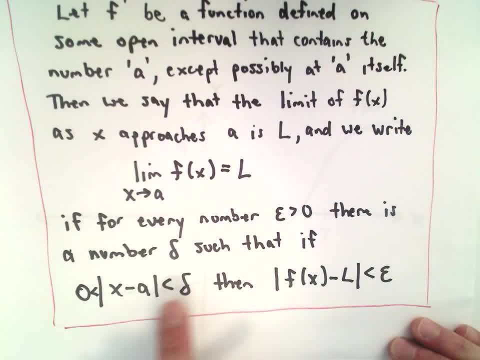 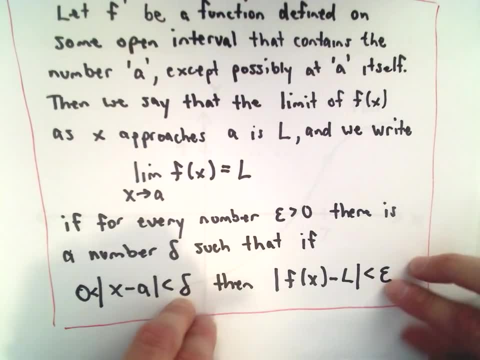 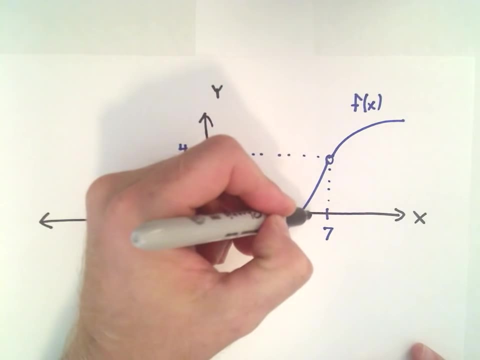 This stuff at the bottom says: hey, if you've got a number close to a, then the value of the function should be close to l. Okay, that's all it's saying. So let's look at this example. Okay, so in this case, right as we get closer, if we take a value closer and closer and closer to seven, 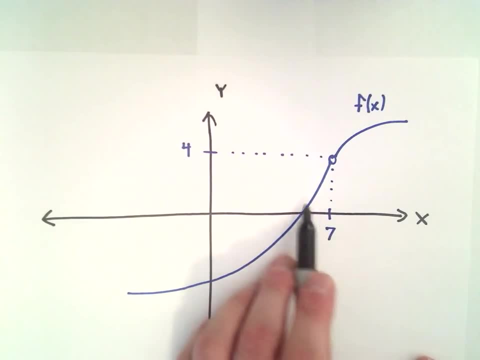 closer whether we come from the left or the right. it says the function takes values closer and closer and closer to the y value of four. So again it said that it didn't have to be defined. It's defined in a itself. 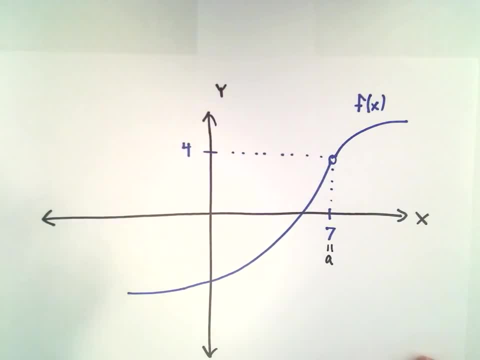 You know, in my case this is my a value. It's seven. And notice the function. I put an open circle there. It could be filled in. It doesn't have to be, And my limiting value here is four. So we have the limit as x approaches a, which in this case is seven of f, of x. 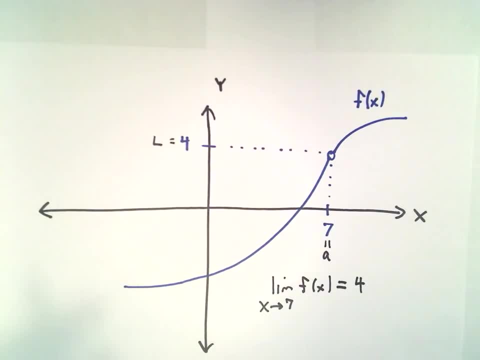 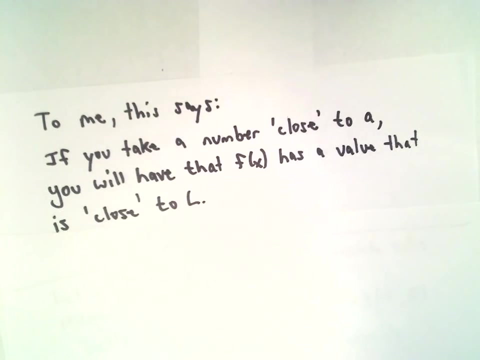 That equals four. Okay, I'm sure you know at this point, if you're dealing with the definition, I'm sure you've seen this notation and have seen it. You've seen finding limits from graphs, So okay, So again, again, all that definition to me is saying it says: if you take a number close to a, 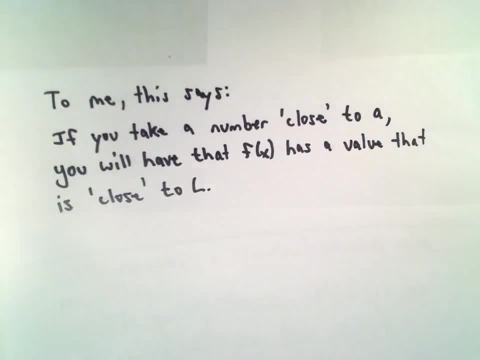 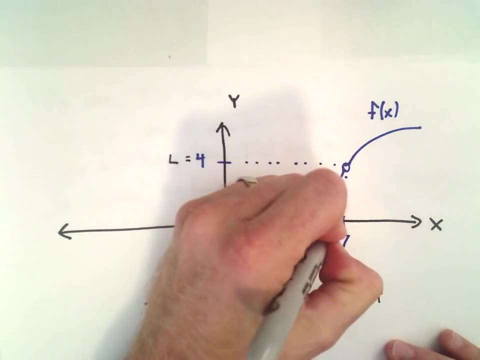 you'll have that f of x has a value that is close to l Again, right, if we take a value close to a close to seven, right? so maybe I take some little open interval here If I take numbers close, close to seven. well, you know, if you look at, okay. so if I follow up here, 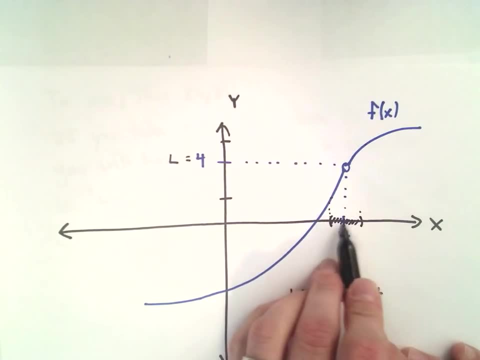 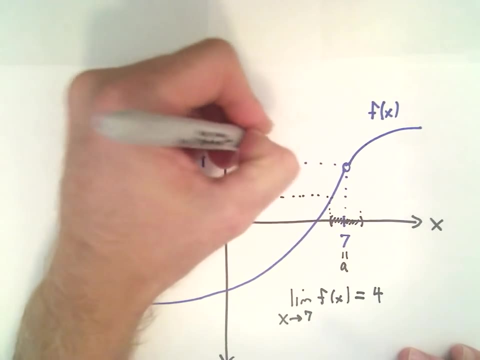 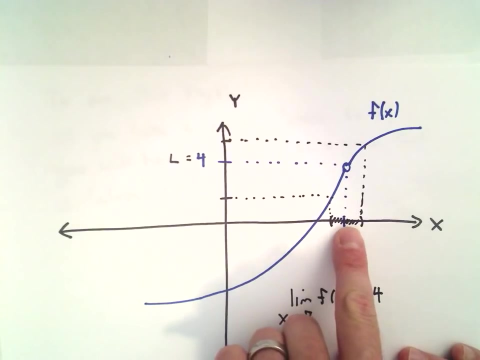 and if I follow up here, if I take numbers in this little interval, you know, if my graph is relatively correct, if I take numbers that are close, that are close to a. so I'm taking numbers in this little open interval. 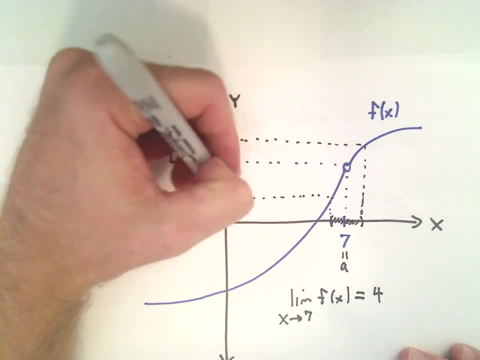 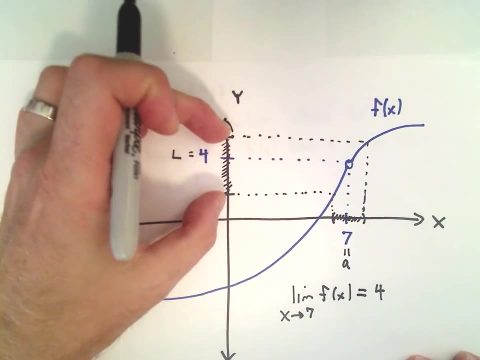 I'm getting values on the y-axis that are, you know, right. I'm getting values on the y-axis that are, you know, relatively, again, close. We haven't made close precise, but you're getting values that are going to be somewhat near the limiting value, in this case, of four. 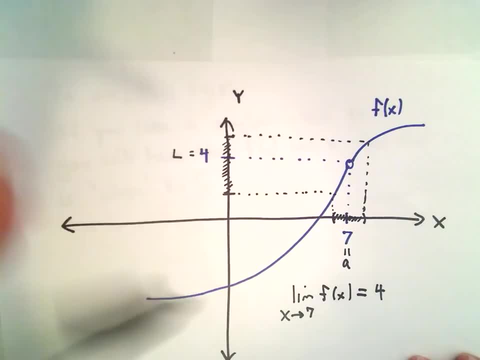 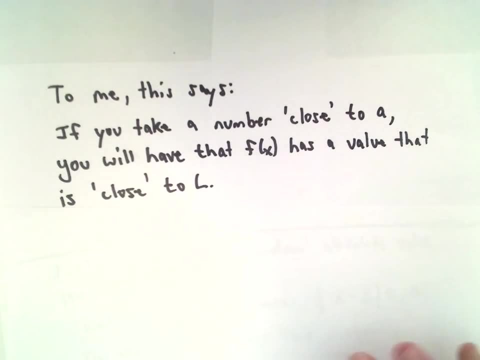 Okay, so that's the idea. Take a number close to seven, you'll get some number. hey, you'll get some number on the y-axis that's relatively close to four. That's all we're trying to do. Okay, that's all we're trying to do. 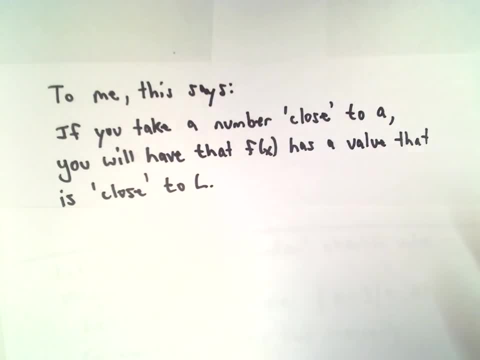 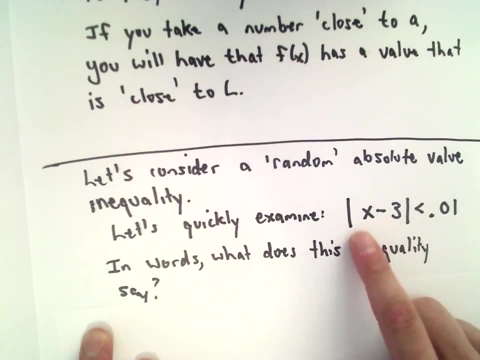 It says: if you take a number close to a, you're going to have a value that's close to l. Let's look at just a random absolute value: inequality. Let's think about this inequality: the absolute value of x minus three, less than .01.. 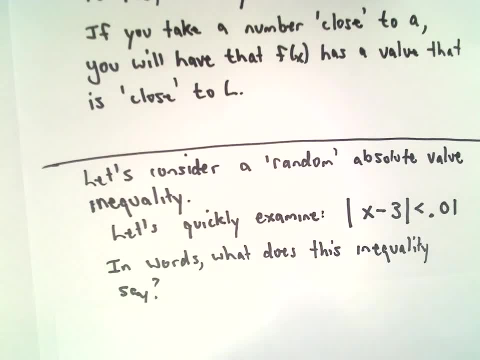 You know in words. what does this say? What does this inequality mean to you? Does it just mean you know some random symbols? To me? I can put it in words, but let's look at solving it real quick. 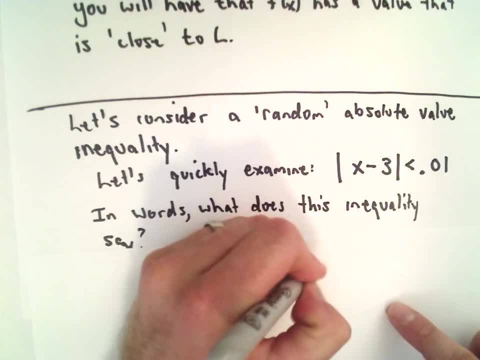 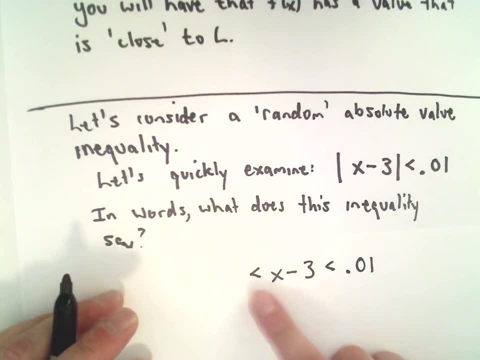 So, if you recall, to solve this type of absolute value inequality, okay so we just remove the bars. Then we also make an inequality. We're x minus three is greater than the negative of that number, so negative .01.. Okay so the solutions to the absolute value of x minus three less than .01, we'll get the solutions by solving this compound inequality. 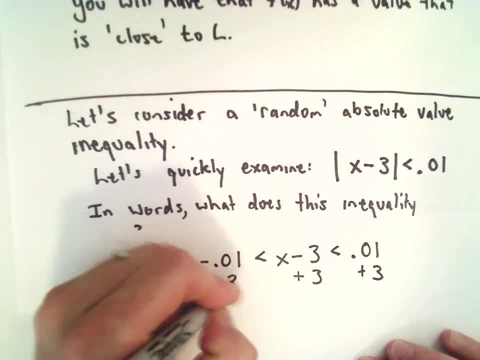 So to do that, we'll just add three to both sides. Well, positive three minus .01, that's going to be 2.99.. .01 plus three, that's going to be 3.01.. So again, bear with me. 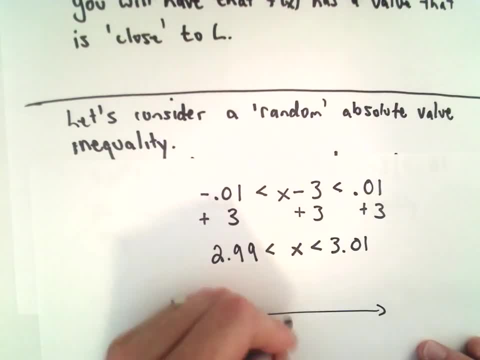 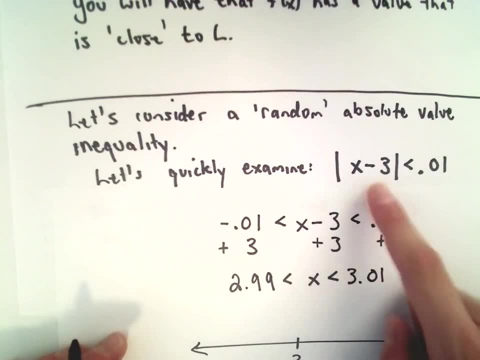 This video is going to take a couple minutes because I think this definition is a little can be a little confusing, So okay. so there's our number three. It says values that are going to satisfy that inequality. it says we need numbers that are greater than 2.99 but less than 3.01.. 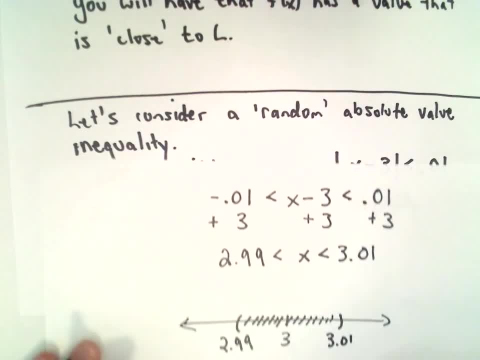 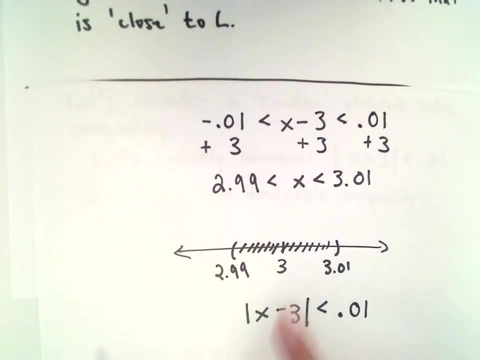 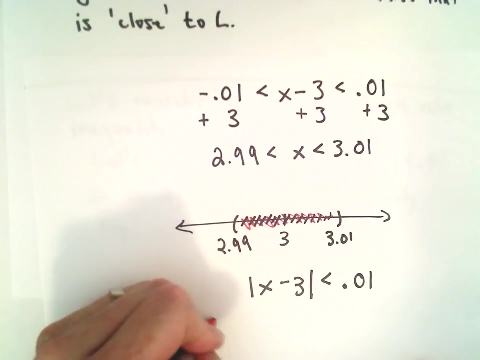 So any number inside of that interval, any number inside of that interval, is going to satisfy this inequality. Well, again, in words, in words, what's happening To me? well, we're getting, we're getting numbers, we're getting numbers that are, again, quote, unquote, close to the number three, right. 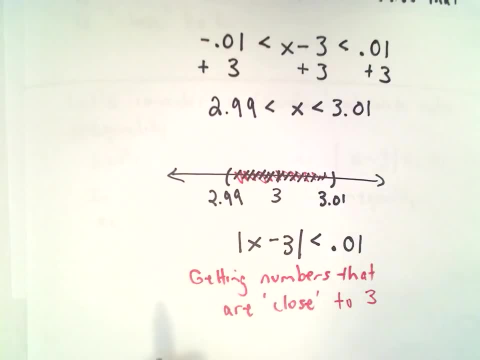 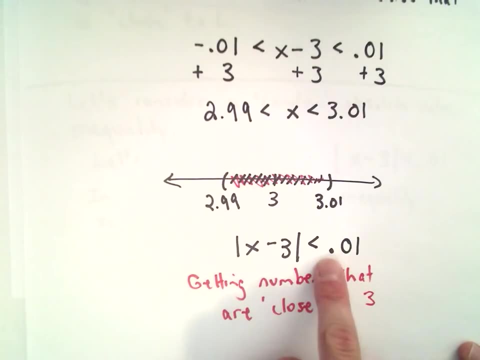 We're getting numbers that are within .01 of the number three. So that's all this absolute value In a quality saying. it says, hey, you're going to get numbers that are within .01 of the number three. You know, if I make this number even smaller- .001 or .0001, the numbers that are going to work are going to be in an even smaller interval. 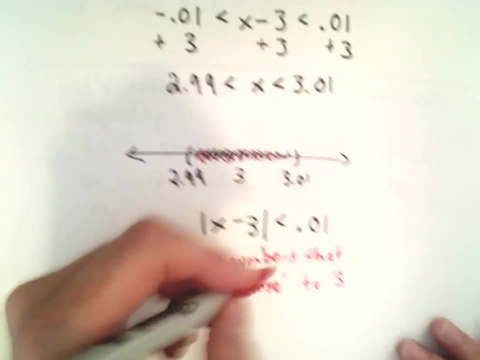 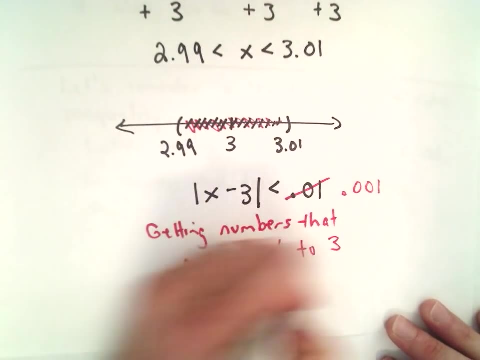 They'll be even closer to the number three, right? If we use, say, instead of x, instead of using .01, suppose we use .001.. Well, in that case, there's my number three, And what would it be? 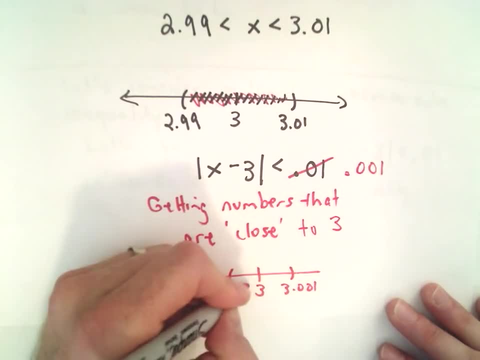 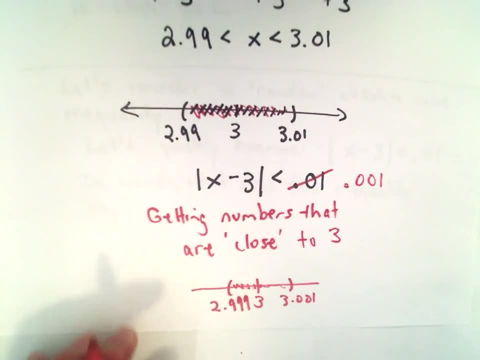 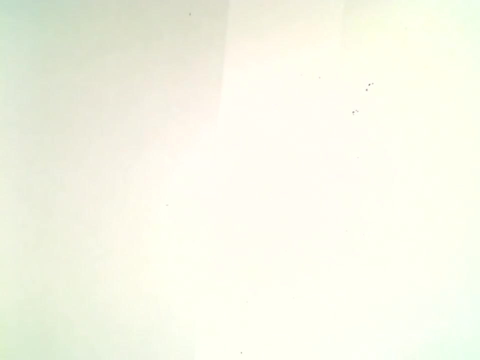 2.9, 2.999 looks like it would work. We're going to get numbers in an even smaller interval that are going to satisfy the absolute value inequality. Okay, so this is the idea. Back to the definition. So if this number, delta, is small, this is like my x, you know, minus three, less than three. 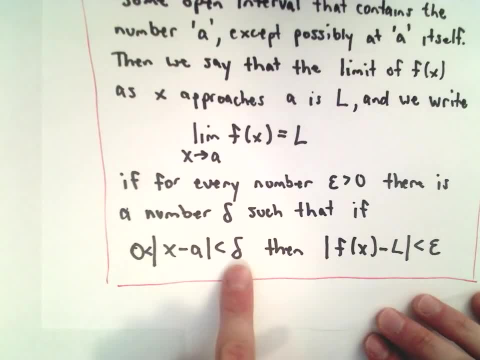 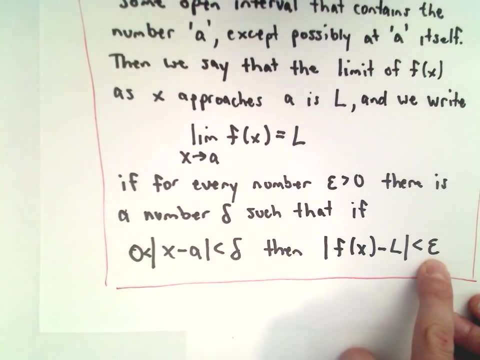 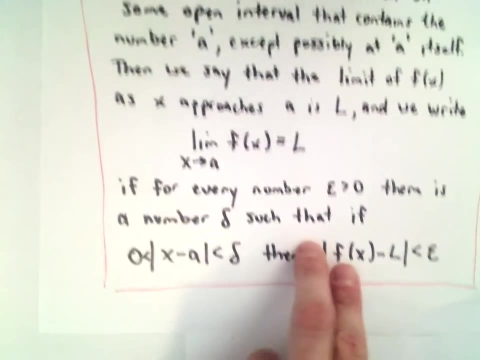 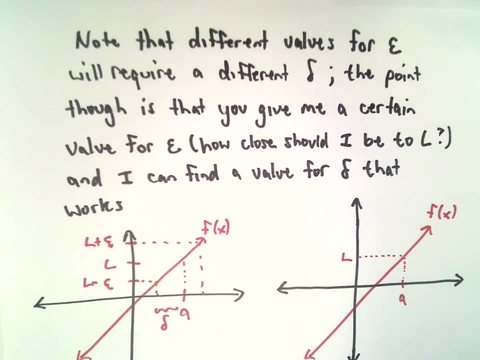 Okay, This is going to be less than .01.. If delta is small, you're going to be really close to that number a, And if epsilon is really small, you're going to get y values really close to that number l. Okay, so that's all. this definition is trying to encapsulate this notion of closeness. 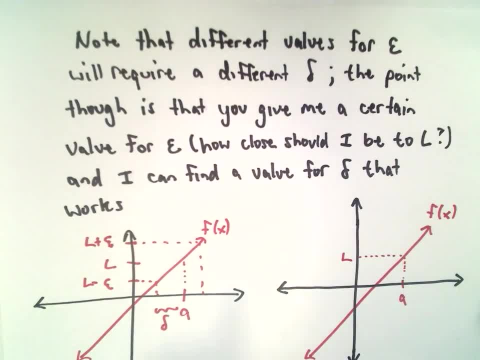 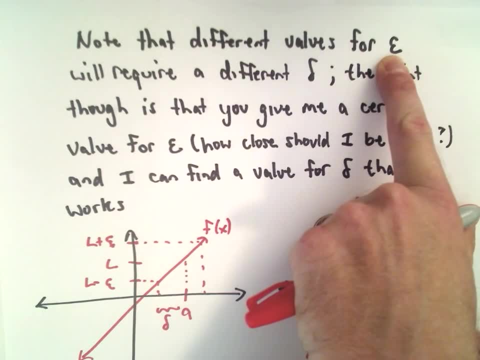 So a different thing to point out as well. This is the last thing I want to point out here, before we actually start using this definition. You know, depending on the value you give me for epsilon, you're going to need a different delta. 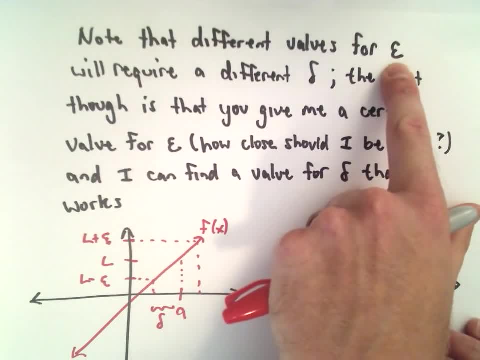 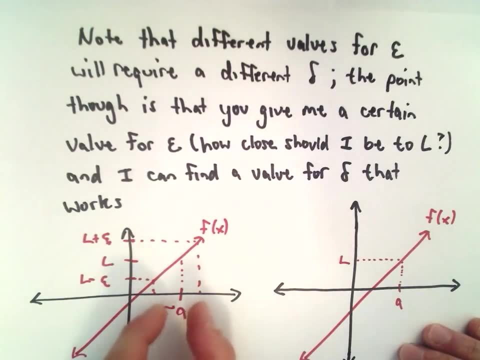 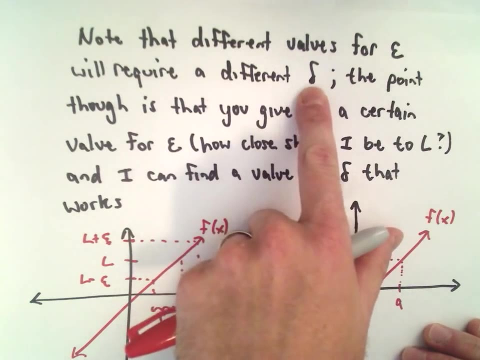 But that's the whole point. You specify this epsilon, You tell me how close you want me to be on the y-axis And I'll tell you how close you need to be on the x-axis. And if you want me to be really close, maybe I've got to find a really small delta. 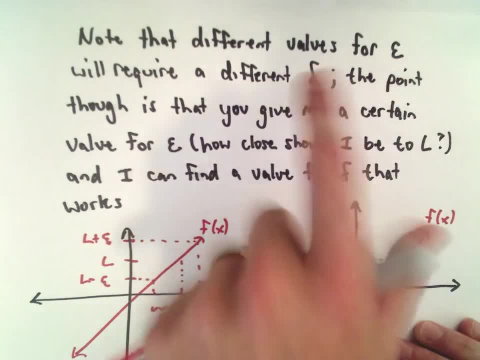 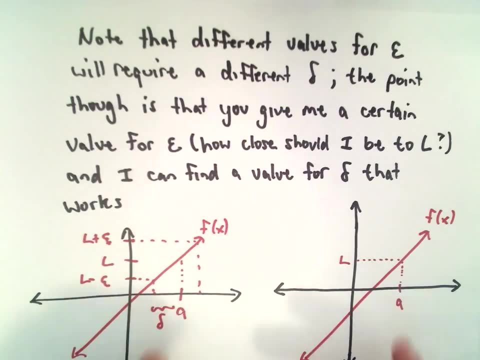 But the point is, you tell me how close you want me to be. I can always find some interval that works. If that happens, then we say the limit exists. So again, intuitively, if epsilon is a little bit bigger, I've got a little more wiggle room on the y-axis. 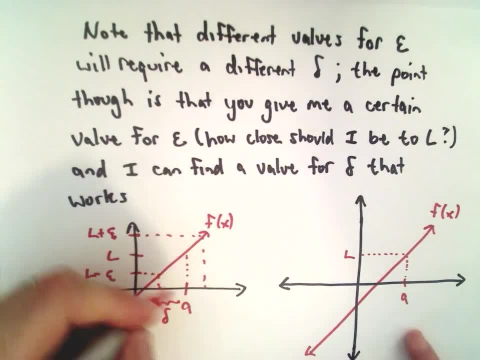 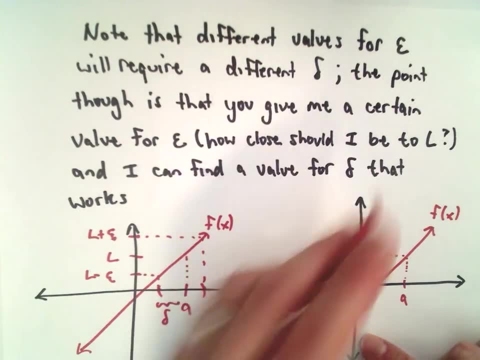 which means around my a value again, I'm going to have a little more wiggle room as well. Okay, I can probably take a larger interval If I want my epsilon to be a really teeny, tiny number, which means again, I want to be really close. 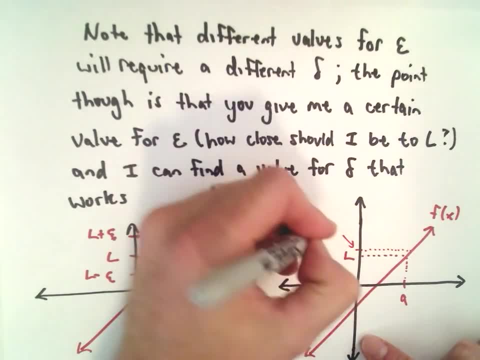 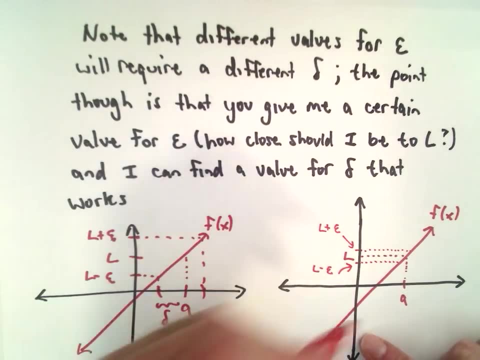 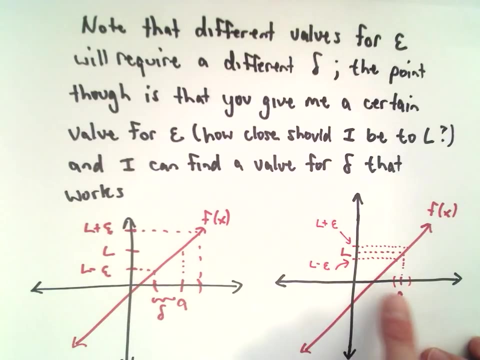 so maybe this is the value l plus epsilon and this is going to be the y value l minus epsilon. Well, now I'm going to need an interval that's smaller. Intuitively, most of the time you're going to have to be closer. 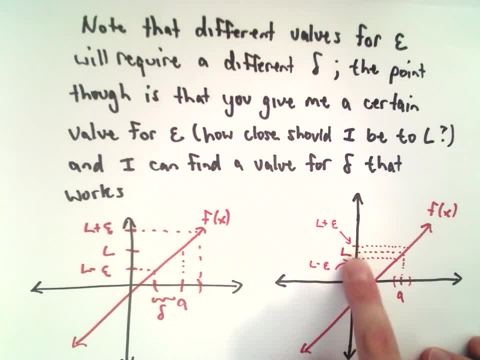 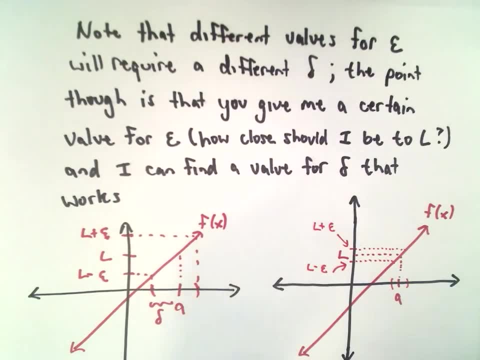 If you want me to be close on the y, if my range of numbers that work on the y-axis is small, you're probably going to need a smaller interval around a. So that's all That's what this definition is trying to say. 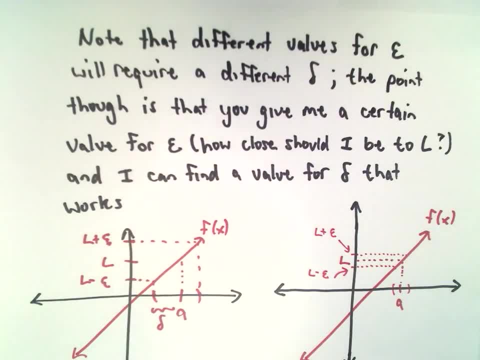 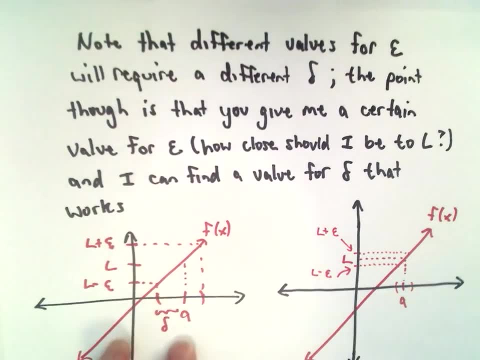 It's trying to encapsulate this notion of closeness. That's all it's doing. So, again, if you got through this video and it made perfect sense to you, hey, I am super impressed with myself. I would be shocked if many people got it on a first watch. 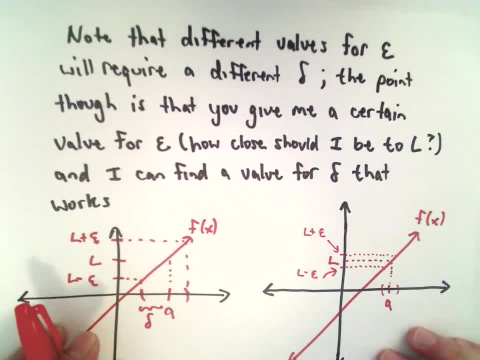 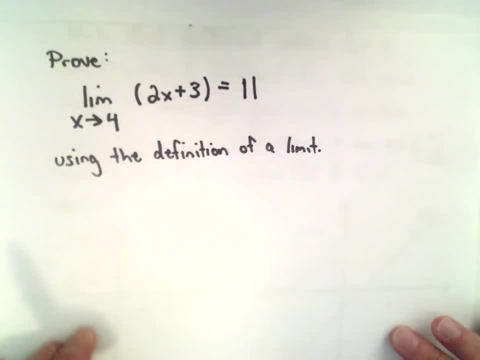 But again, just think about this notion of closeness and what limits mean intuitively to you. And that's all those absolute value inequalities are talking about. So in a couple videos, in another video, I'm going to prove the limit as x approaches 4 of 2x plus 3 equals 11 using the definition.